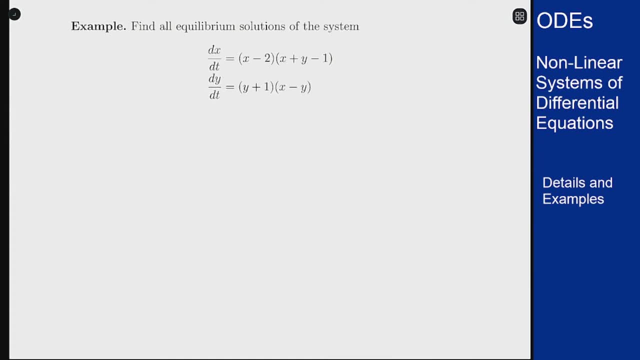 In this video we want to find all equilibrium solutions for a given non-linear system of differential equations. Equilibrium solutions for these equations mean that they are places where the solution does not move anywhere and stays constant. So for a system like this means we're. 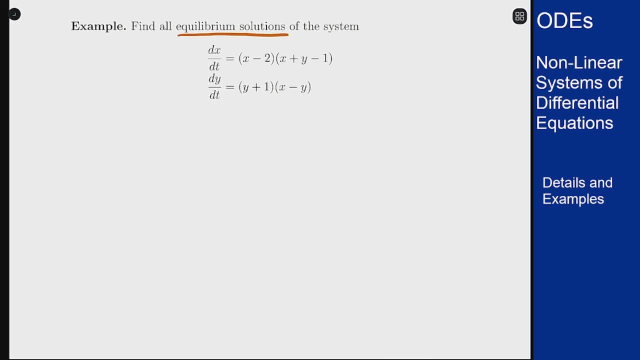 looking for a place where both derivatives are zero. So we want that both dx dt equals zero and dy dt equals zero. Based on our equations, we know that dx dt is given by x minus two times x plus y minus one. we want that to be zero, as well as y plus one and x minus y equaling zero. 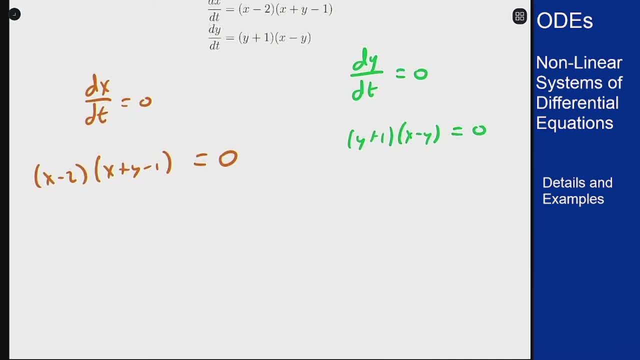 So in the first equation we see that we have two factors here, so we can split these two things up into either x equals two, so that x minus two equals zero, or x plus y minus one equals zero, which we'll leave like that for now. For the second equation, for dy dt being zero, we 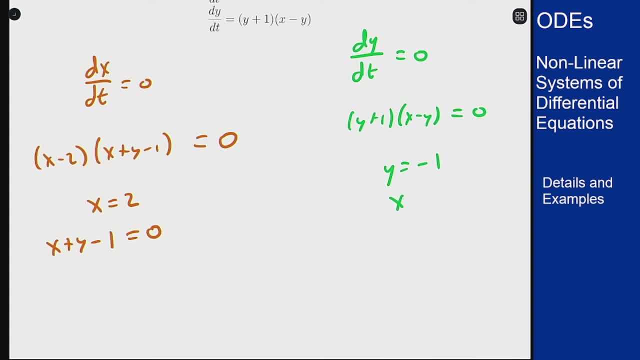 get that either y equals minus one or x plus y minus one equals zero. x equals y, because x minus y equals zero. Now, from this, we want each of these to be true at the same time, so we want this to be an and between these. between then, you pick one equation from the left. 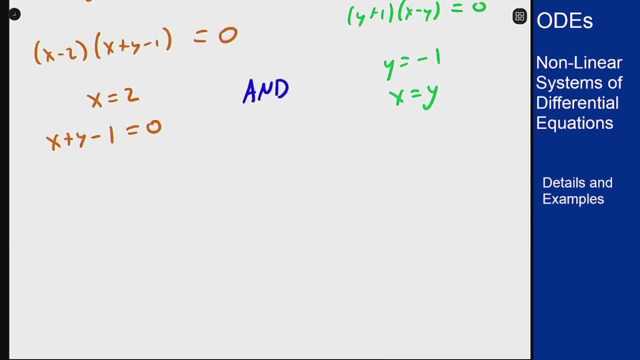 and one from the right to be true at the same time. So for one point we could pick that x equals two and that y equals negative one. give me the point two, comma minus one. We could put x equals two and x equals y, which gives me the point two for x, and then x equals y. y is also two We could pick. 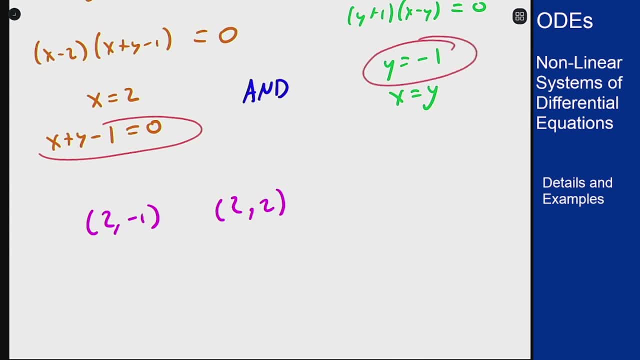 x plus y minus one equals zero and y equals minus one. that will give me the point minus one for y and in terms of x, if I plug minus one into here, I will see that I get x minus one. minus one equals zero or x equals two. that puts the two in here. 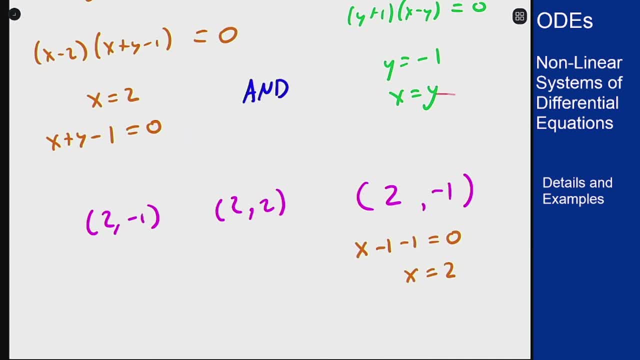 If I pair up the bottom two we get that x plus y minus one equals zero and x equals y. just to replace the x and the equation by a y, to give me y plus y minus one equals zero or y is one half, that's two y equals.